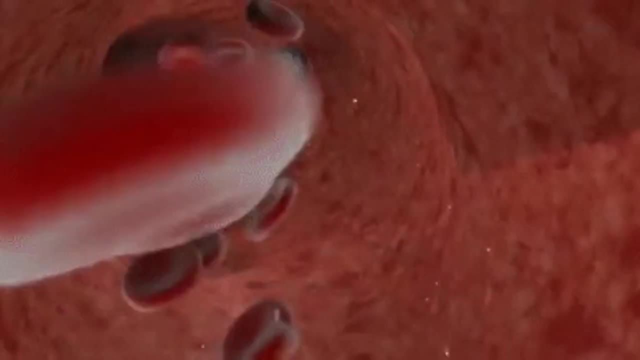 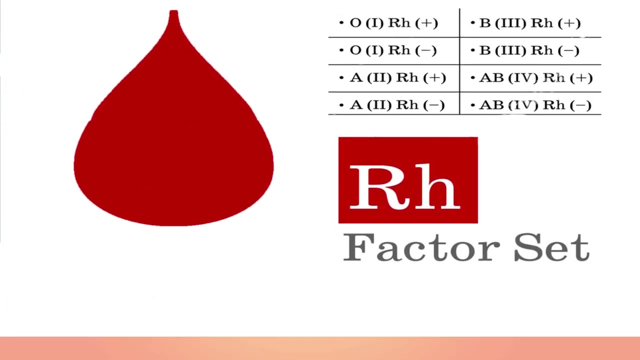 Antigens are substances that activate an immune response and control what enters and exits a cell. Each blood group can be either positive or negative, resulting in eight possible blood types. The plus or minus part of a person's blood type is determined by the presence or absence. 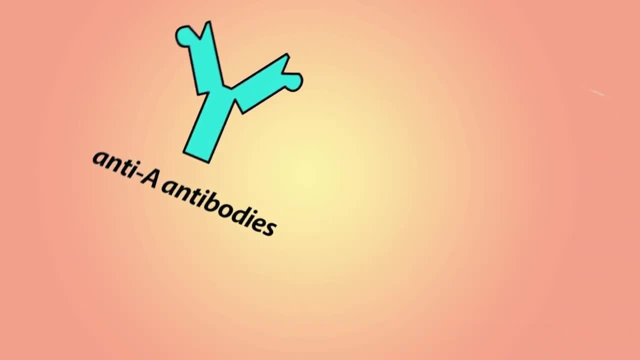 of the third antigen called the Rh factor. Our bodies can handle blood without the presence of an antigen that we usually have, but cannot handle the introduction of a new antigen into the circulatory system. That's why people with zero minus blood are known as universal donors. 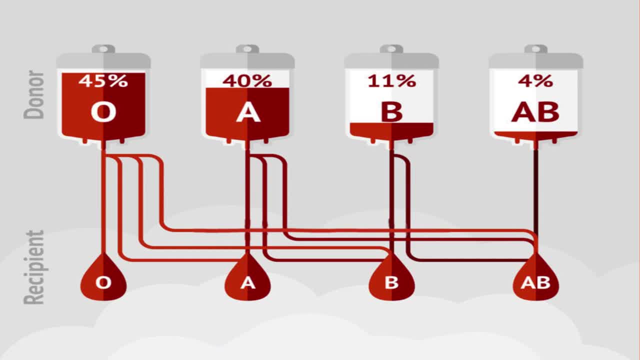 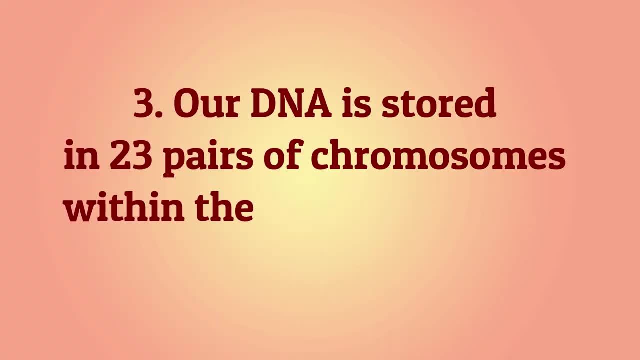 Anyone can use zero minus blood. People with AB plus blood, on the other hand, are universal recipients. They have every antigen in their blood already. Our DNA is stored in 23 pairs of chromosomes within the nucleus of every cell in our body. 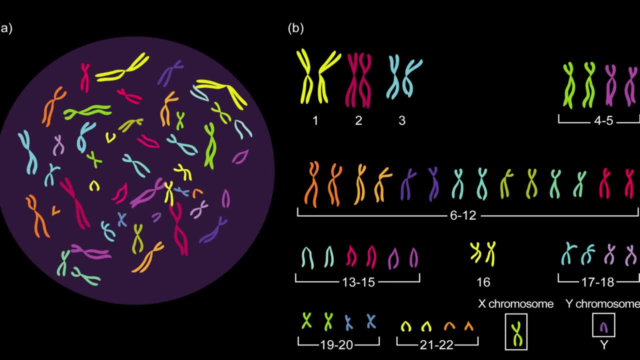 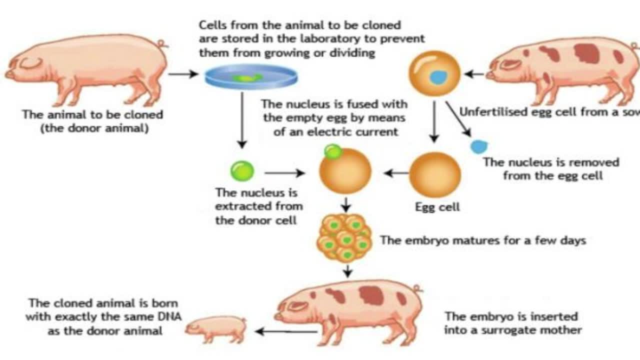 Each cell has a full set of chromosomes, which contain all the genetic material needed to determine the makeup of our entire bodies. That's why cloning of animals can be done with just one cell. All the genetic material that defines us is inside each and every cell of our body. from. 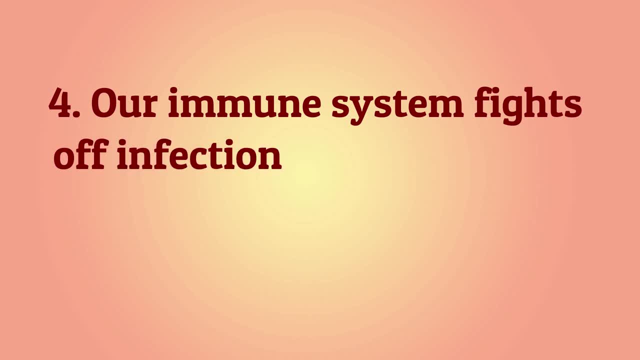 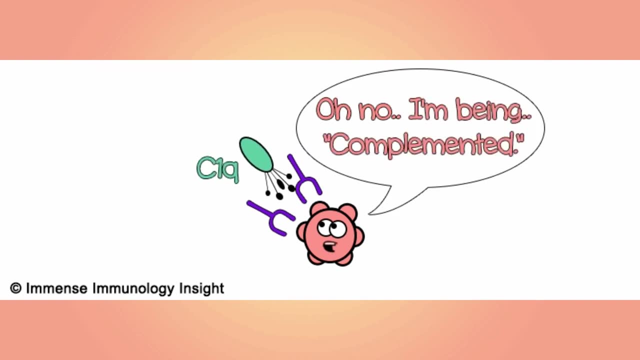 our hair follicles to toes. Our immune system fights off infection mostly through the use of antibodies and macrophages. Antibodies actually fight infection by killing the virus or foreign bacteria, while macrophages are white blood cells that surround and contain the foreign cells to prevent the spread of. 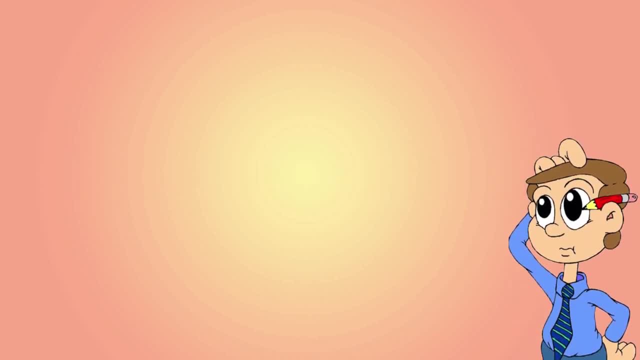 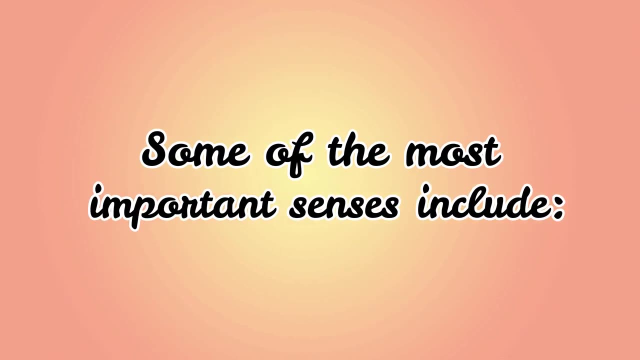 disease. We have more than five senses. While we typically think of the traditional five senses of touch, taste, hearing, vision and smell, our bodies can actually sense many other things. Some of the most important senses include balance, temperature, proprioception, spatial. 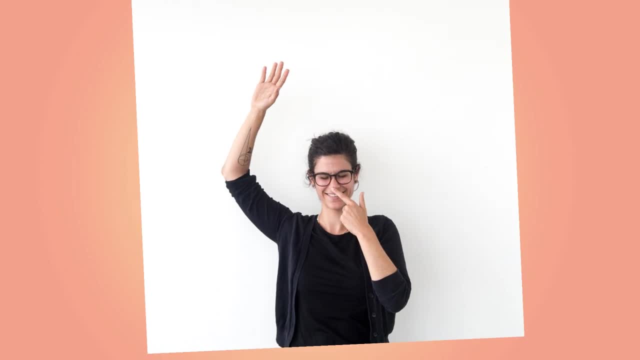 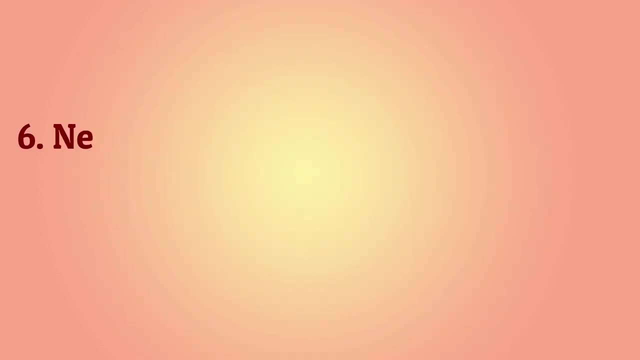 body awareness and memory. The most important sense is the sense of smell, which is the most important sense of body awareness, aka why you can touch your nose with your eyes, shut Pain which is associated with its own organ, Taste with your tongue, smell with the nose, or sensory receptor. 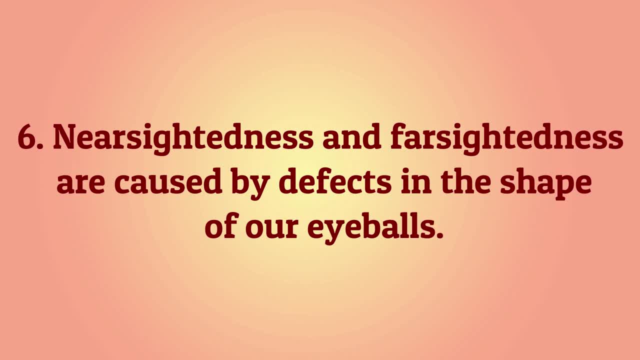 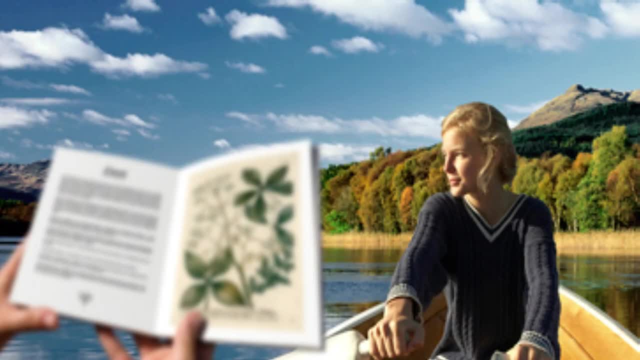 Nearsightedness and farsightedness are caused by defects in the shape of our eyeballs. Nearsightedness, or myopia, is caused by a greater curve in the cornea of the eye or by an elongation of the eyeball. 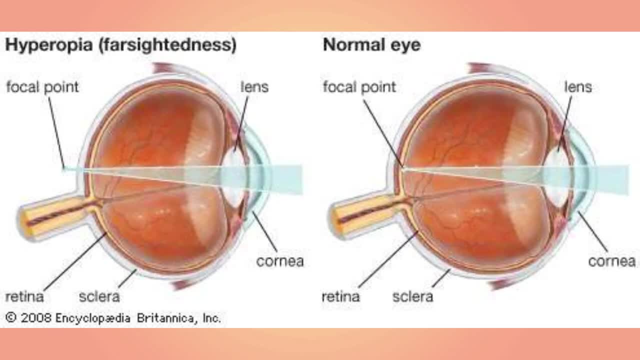 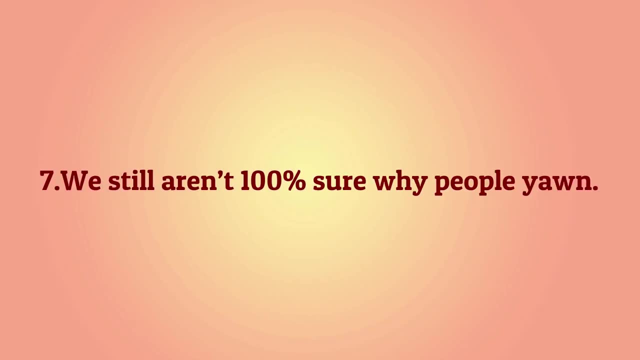 Farsightedness or hyperopia is caused by a corneal curve that is too small or by having a short eyeball. Some evidence indicates that nearsightedness is genetic. We still aren't 100% sure why people yawn.